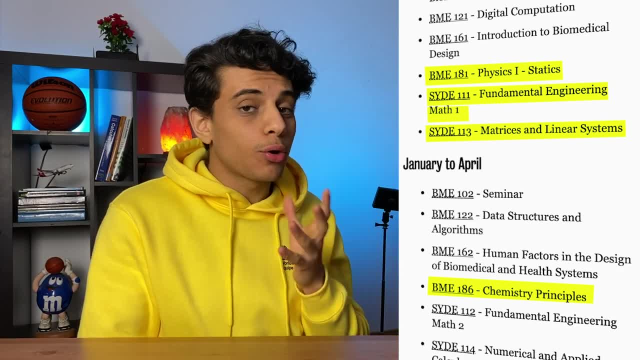 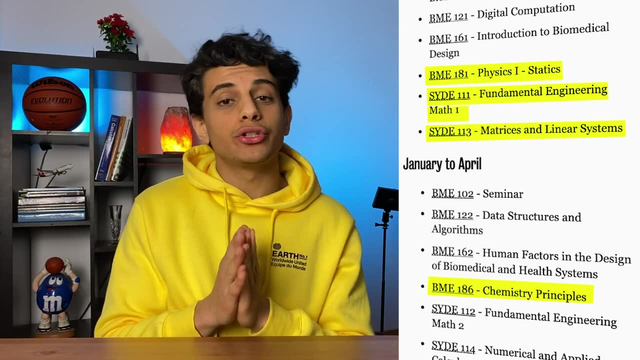 chemistry, calculus, linear algebra. These are like fundamental courses in engineering because you know, the purpose of first year engineering is to get everyone caught up on the fundamentals. An interesting course that biomedical engineering students take is data structures and algorithms. This course teaches you the basics of software engineering. So 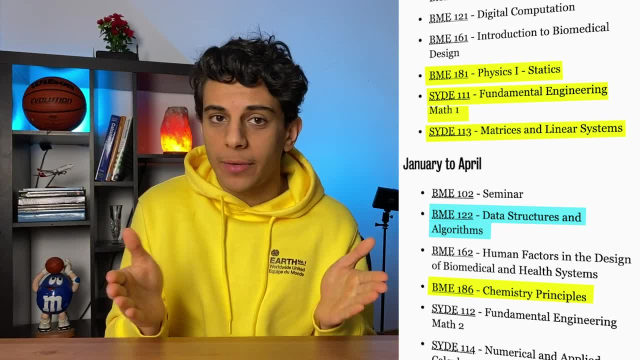 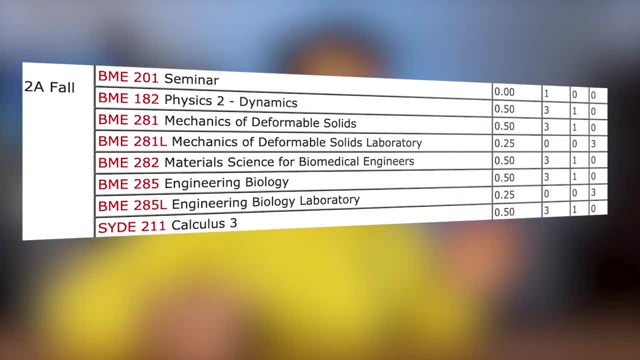 although you're studying biomedical engineering, there are still students who graduate from biomedical engineering and can work as software engineers. Once your first year is over, you'll move on to your second year and you'll be taking these courses In 2A. you will notice that you 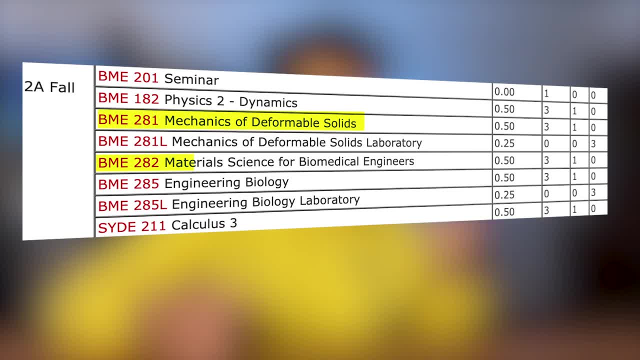 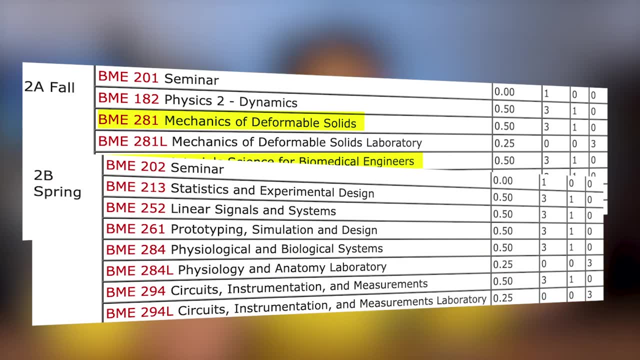 have some mechanical engineering courses like mechanics of the vulnerable solids and material science. You also have some bio and a bit of math. In 2B you take some electrical and computer engineering courses and some more bio. Then in third year and fourth year you'll be taking more. 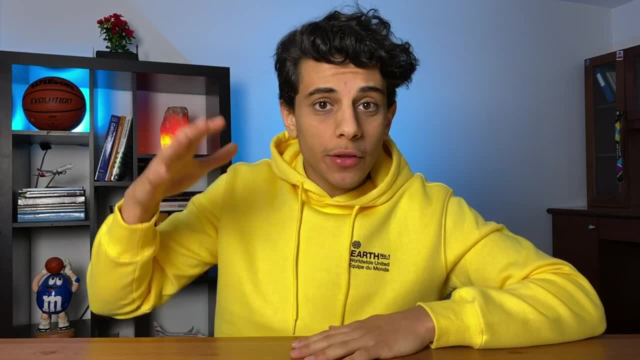 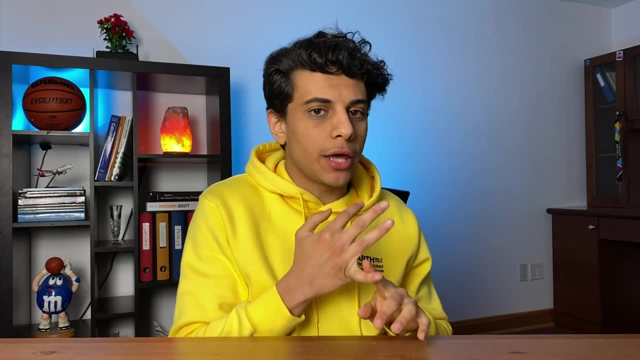 specific biomedical engineering courses. So after looking at all the courses you're expected to take in your biomedical engineering degree, you'll notice you have a lot of mechanical, electrical and software engineering courses with a little bit of biology. This information combined can help you create biomedical systems. 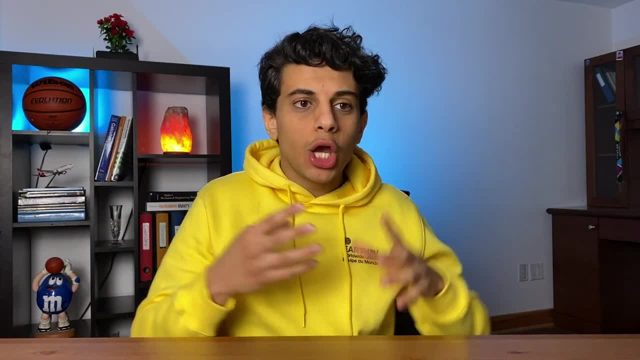 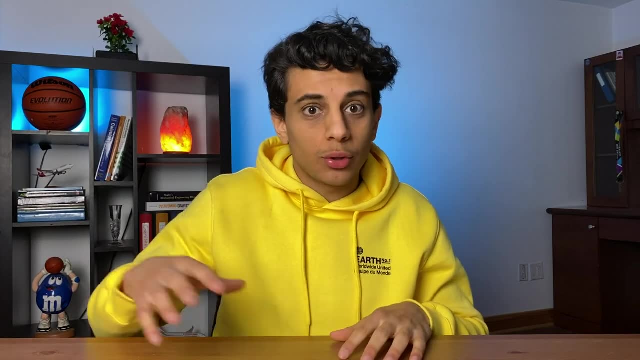 But because you're introduced to mechanical, electrical and software engineering, you can actually end up, you know, disregarding the biomedical engineering field completely after you graduate and just purely working as a mechanical, electrical or even software engineer. So that does give you a little bit of flexibility with that degree. 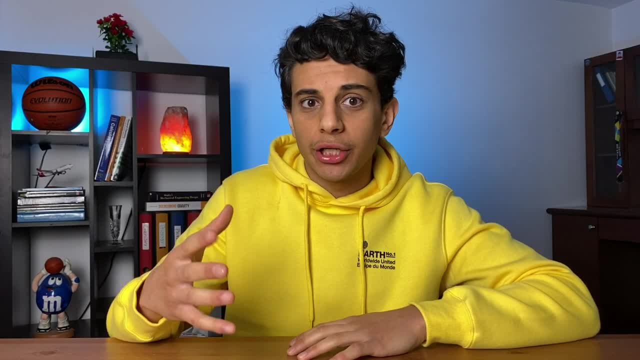 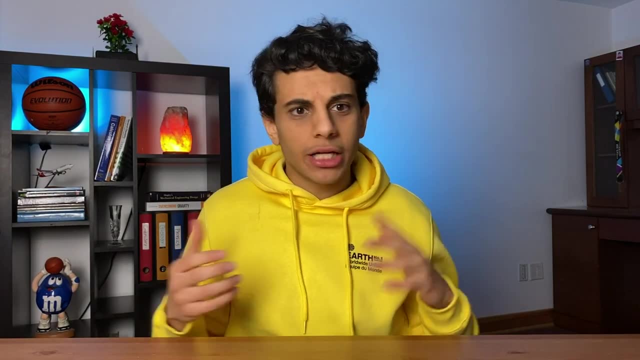 Now let me give you an example of how biomedical courses look like in engineering. So I'm a mechanical engineering student and I'm currently taking a biomechanics course at this semester as one of my technical electives, just because I enjoy learning about it and it seemed interesting And 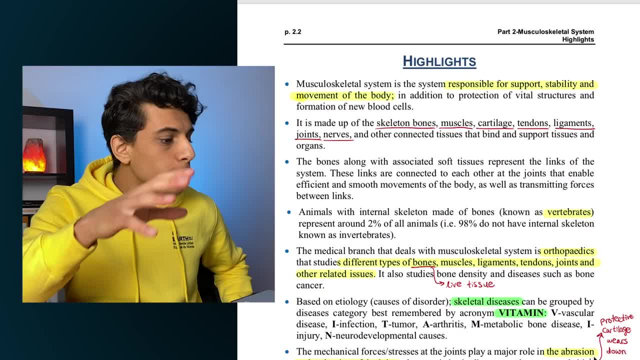 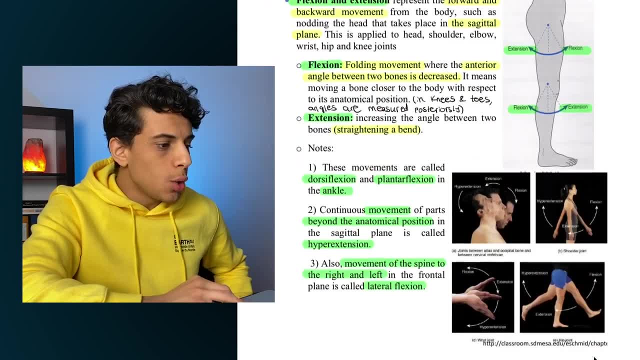 of course it's organized. Now, having a look at the course notes in the assignment, you'll see that the professor first teaches us fundamentals of the human body and human anatomy. you know the type of stuff that you will find in medical courses. We learn about all the different 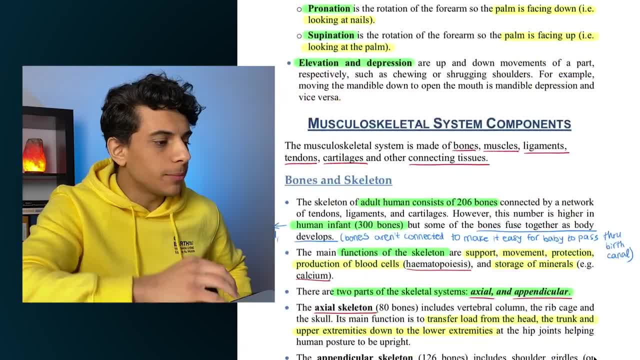 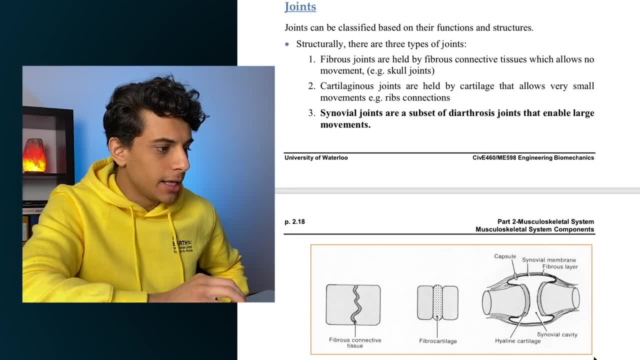 movements in the body. you know what the body can really do, all the bones in the body, as well as the muscles and joints that we have. He'll also teach us about the composition of the bone, as well as bone tissue and a bunch of other stuff like that. Now, once we have that information, 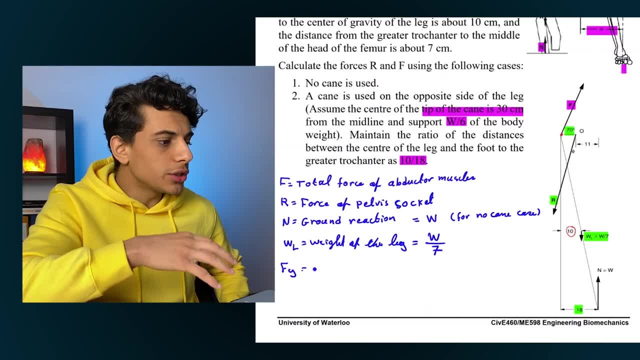 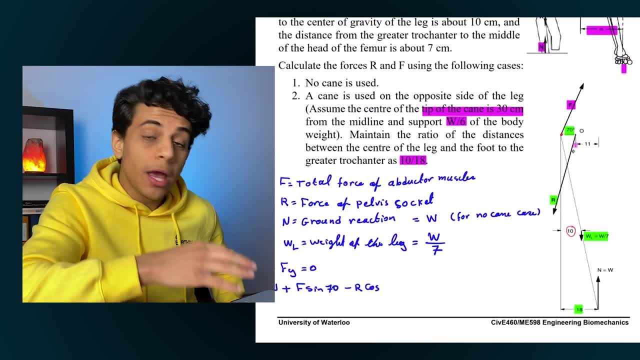 down. you know the type of information that you just memorize. we'll start solving mathematical problems, For example, calculating how the load on your joints and muscles will change based on where you place a cane when walking. Or another example would be using math to determine 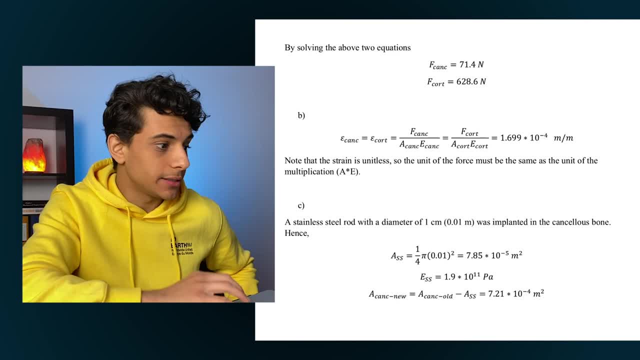 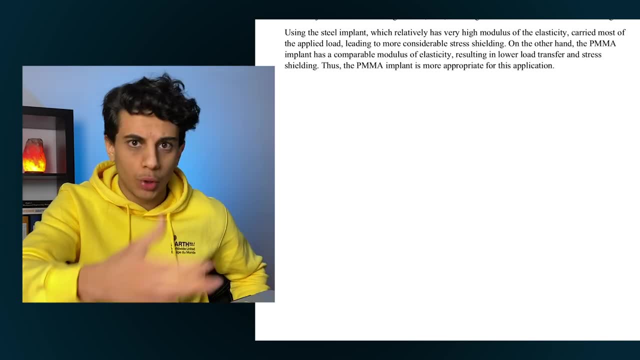 how much load our bones will face if we add implants. So it's basically understanding, like you know, how human body works, and applying math and physics onto it to solve and model real world problems. Once you graduate, you can pursue careers in health design, robotics or research. 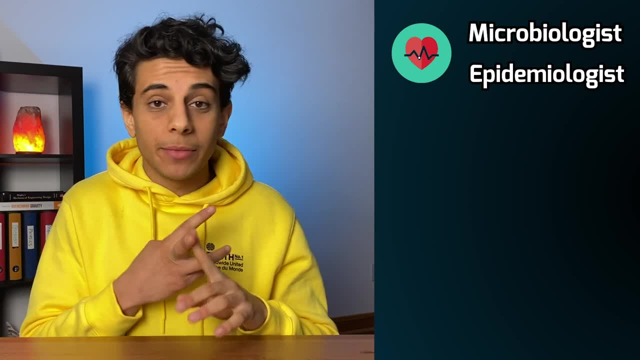 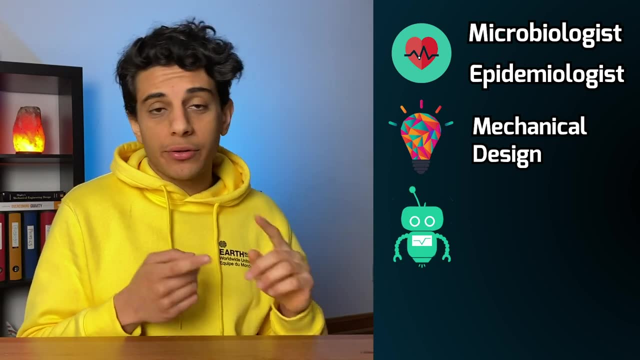 Under the health route, you can get jobs like a microbiologist or epidemiologist. Under the design route, you can be working on the human body. Now I'm going to talk a little bit about the mechanical design of biomedical devices. Under the robotics route, you can be working on the. 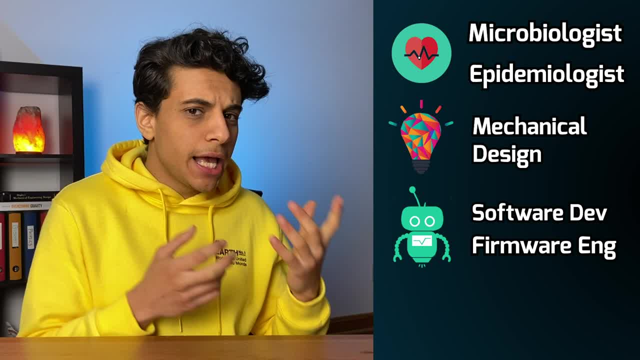 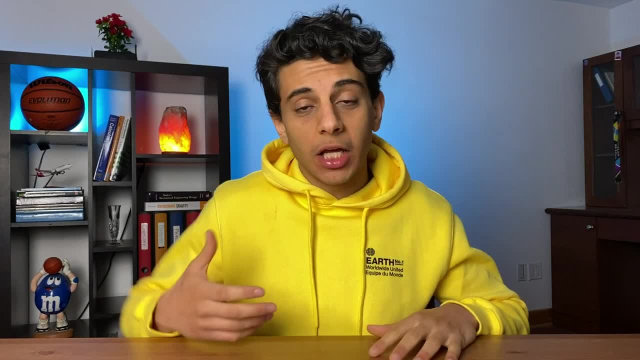 software development or firmware engineering behind these devices. And finally, you can be doing research in labs on future biomedical technologies. So there is a lot of variation when it comes to the jobs available for biomedical engineering students. So it really depends on what area you're interested in the most. At the end of the day, you should realize. 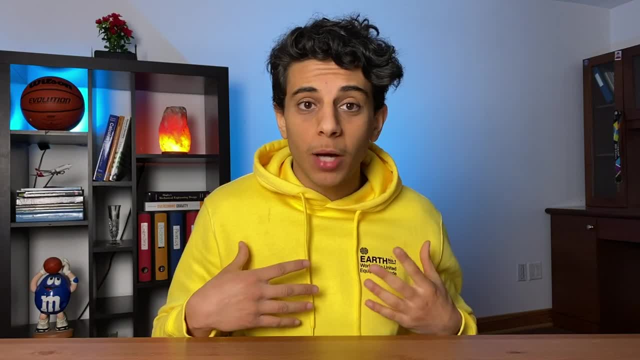 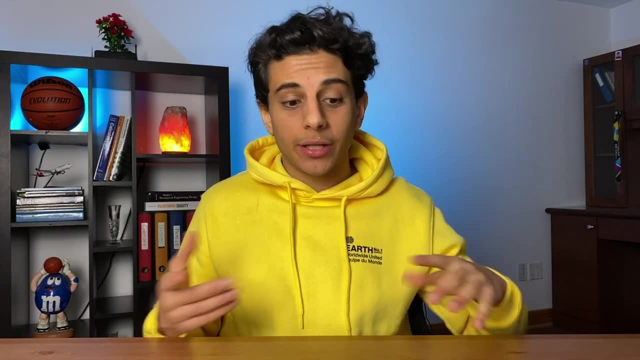 that biotechnology basically involves you creating things that deal with the human body. you know things like artificial limbs, pharmaceuticals, supplements or even biofuel. Your engineering career may lead you to work at a startup tech company, private company, government. 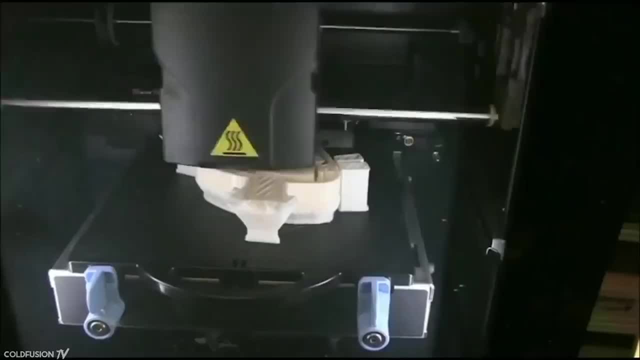 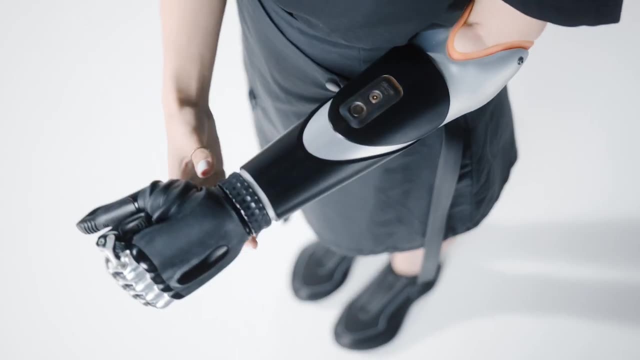 or even clinical labs. You may invent something like bio ink to provide faster 3D printing for kidneys or other organs, or you may work at a company that helps amputees regain mobility by creating high-tech prosthetics. Now, let's be honest, making a positive impact on people's lives. 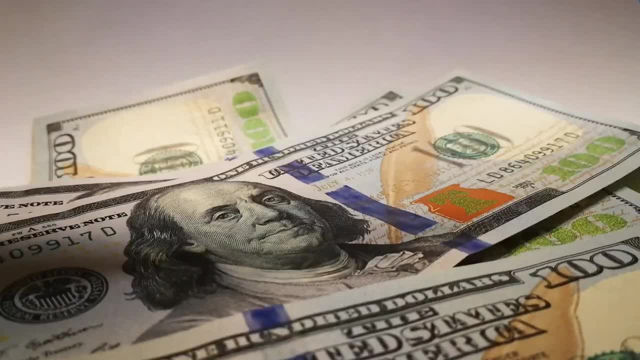 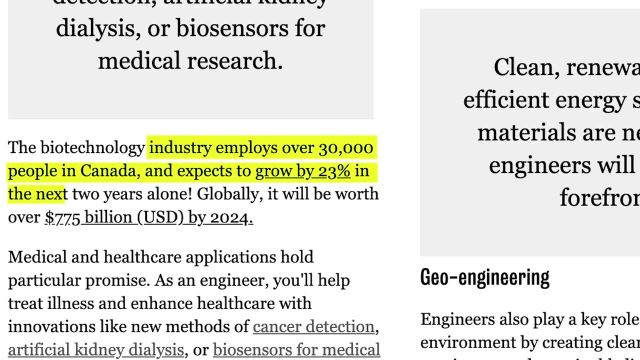 can be a nice and fulfilling career, but money matters, So let's look into how much money a biomedical engineer can make. The industry hires over 30,000 people in Canada, and that number is expected to grow by 23% over the next two years, So there isn't going to be a shortage of jobs in. 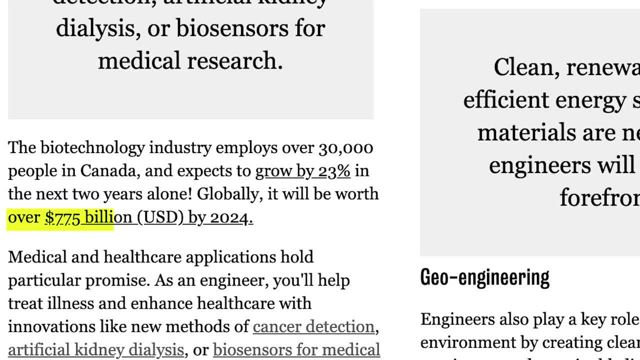 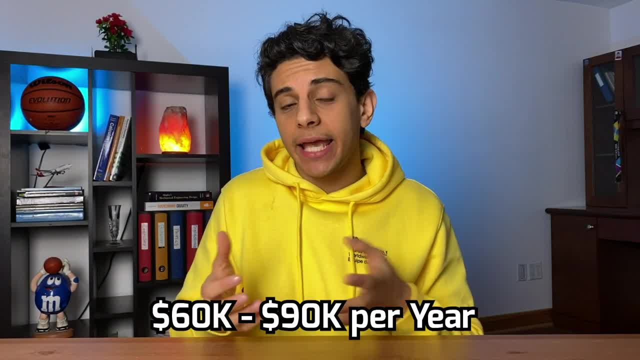 the biotech industry And around the world. the industry will be worth over 775 billion US dollars by 2024.. With that in mind, biomedical engineers can make anywhere between 60K to 90K if they're working in Canada, but that number can be so much higher if they choose to work in California and tech companies, because over there they could be making upwards of $100,000 as an entry-level engineer- Because it's a well-known fact that California pays really, really well, especially at companies. But hey, you can start your own startup with your biomedical engineering knowledge and 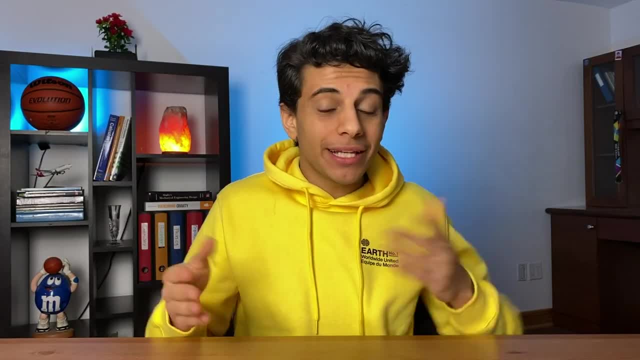 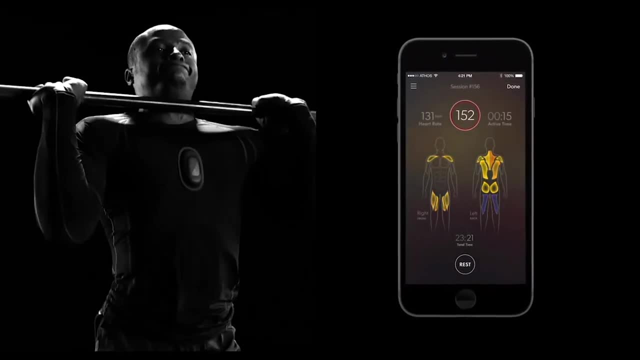 if that succeeds, you could be making millions of dollars. Let me show you an example. Athos was a startup created by an engineer in his final year of his engineering studies. He created smart clothing that measures how hard your muscles are working during your workouts to give you insights. 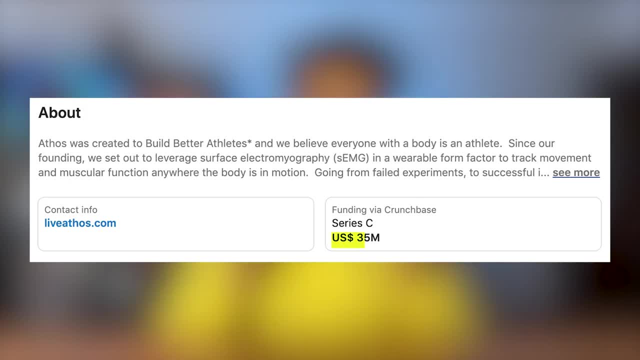 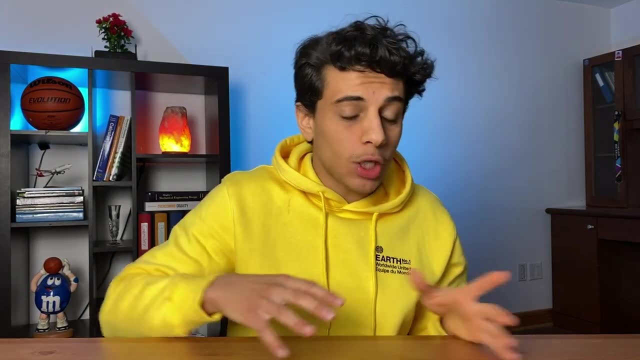 in how your body is performing. This startup raised over $30 million in the past few years and is continuing to do really really well. Anyways, the point of this is that money shouldn't be the deciding factor on what kind of engineering you choose, because it really varies from person. 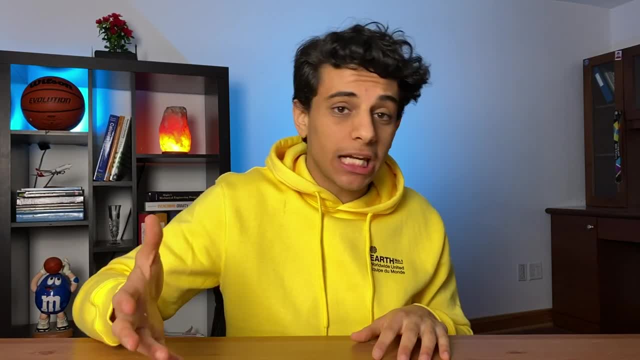 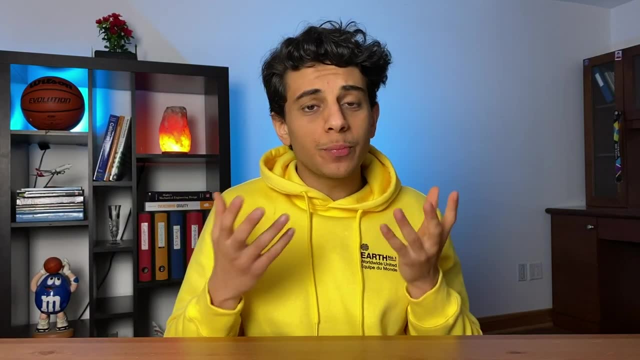 to person and from company to company, and the goal should really be to pick the kind of engineering that you enjoy the most. However, let's say you're interested in the biotech and biomedical industry, but you're not sure whether you should pursue biomedical sciences or biomedical. 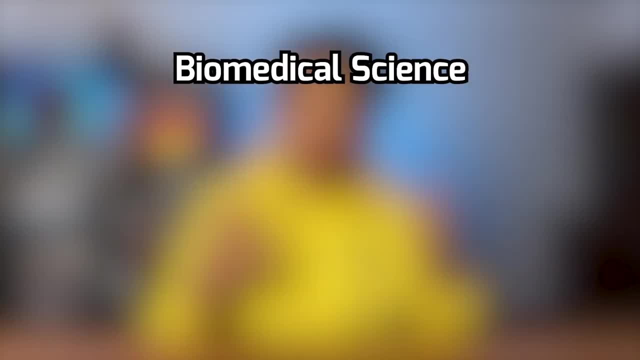 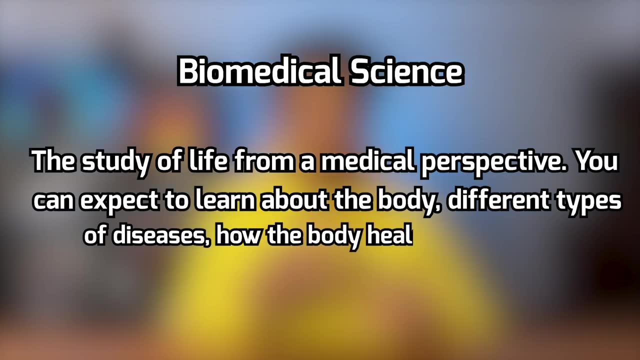 engineering. So let me break down that comparison. Biomedical science involves studying life from a medical perspective. You can expect to learn about the body, different types of diseases, how the body heals itself, genetics and just basically understand how the body works. 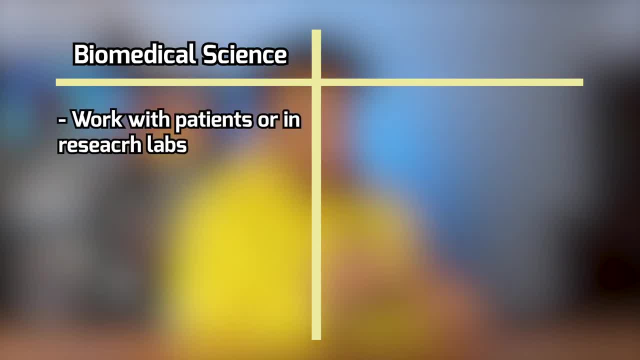 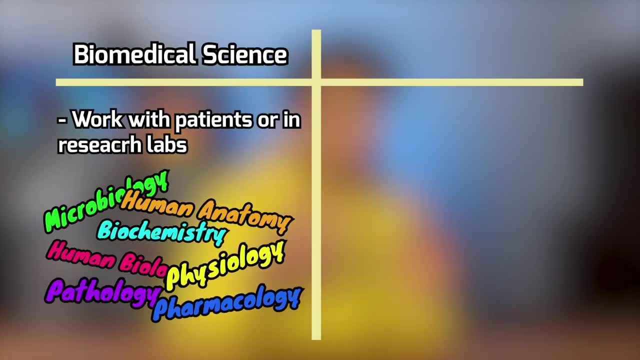 At the job, you'll be expected to deal with patients or be doing research. In school, you can expect to take courses like microbiology, human anatomy, biochemistry, human biology, physiology, pathology, pharmacology, neuroscience, et cetera. 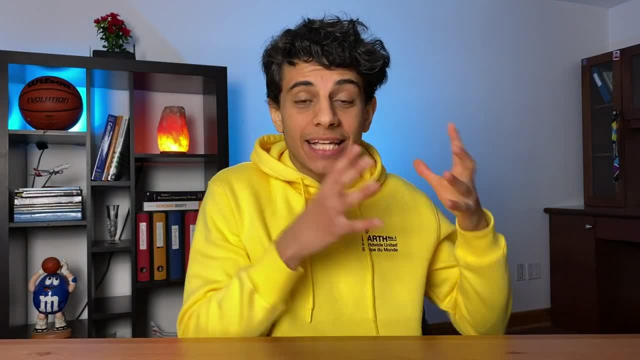 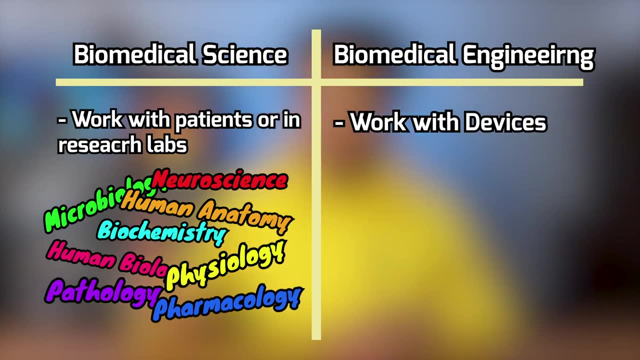 On the other hand, biomedical engineering involves applying the scientific knowledge behind how the body works to design and build medical devices. At the job, you'll be expected to work with devices, and in school you'll be expected to take quite a few biology courses. 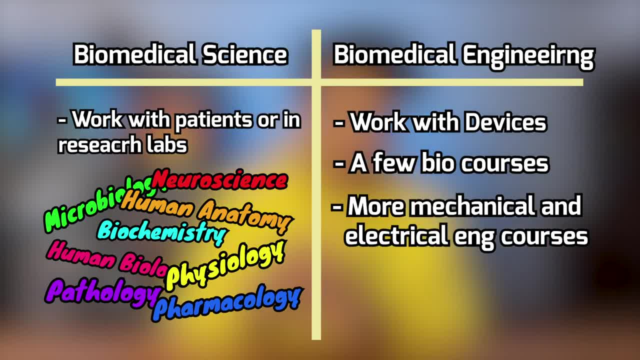 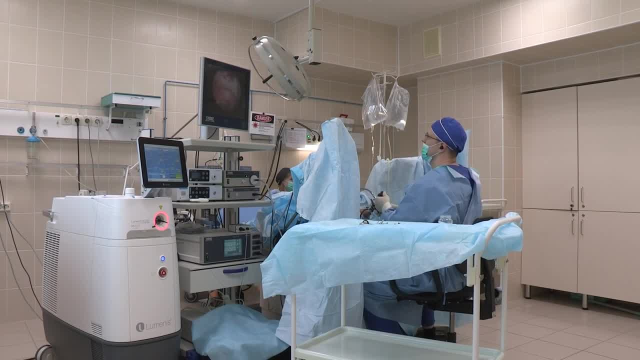 but there'll be a larger emphasis on mechanical and electrical engineering courses, as we talked about earlier. For example, a surgeon will need to understand how the body works to be able to operate on it, But they'll use devices like artificial organs or surgical 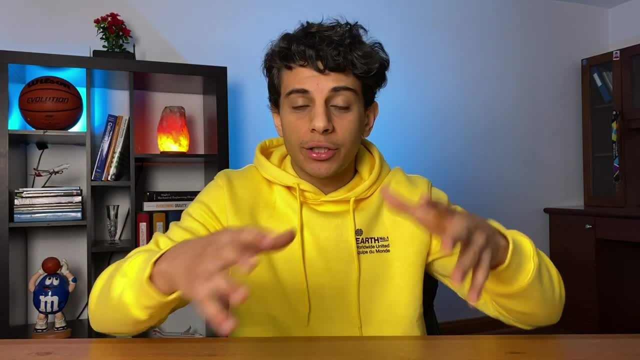 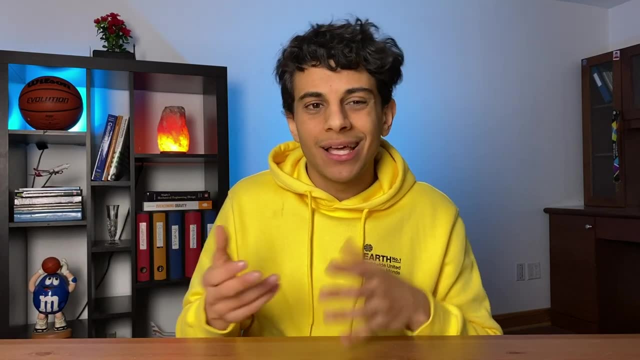 devices that will help them get the job done, and these devices were designed and built by biomedical engineers. Think about it like this: Biomedical science is more theoretical and biomedical engineering is more practical. It's like comparing chemistry and chemical engineering. A common question that may come to mind is if biomedical engineering is a good path. 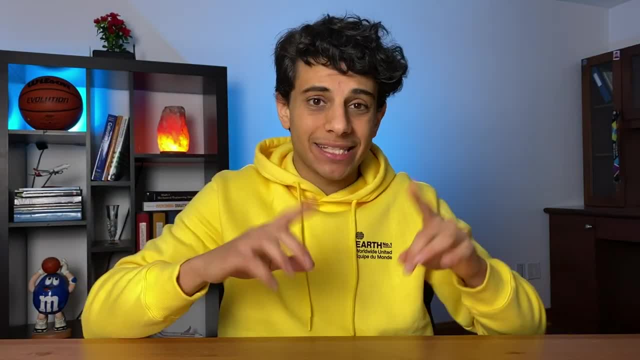 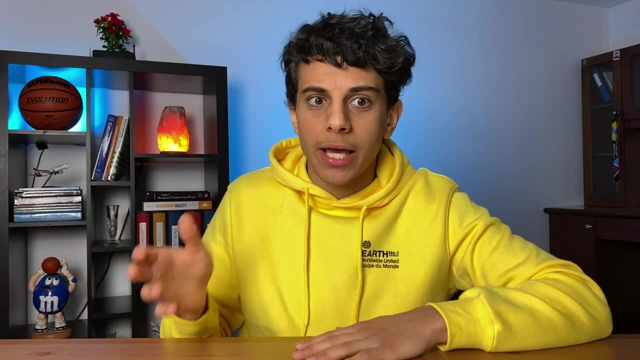 to pursue if you want to become a doctor- Technically, yes, but it can be hard to take all the courses you need to apply to medical school. So if your goal is to become a doctor, then biomedical science would be a much better option than pursuing biomedical engineering. 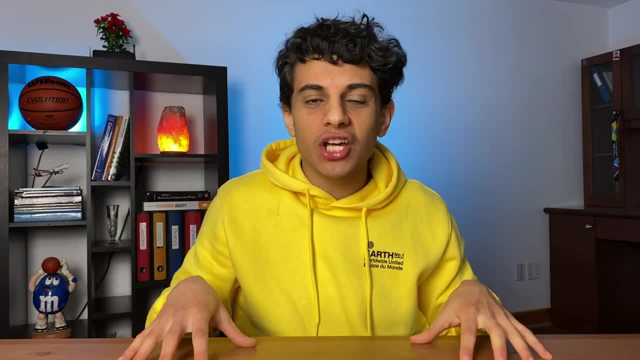 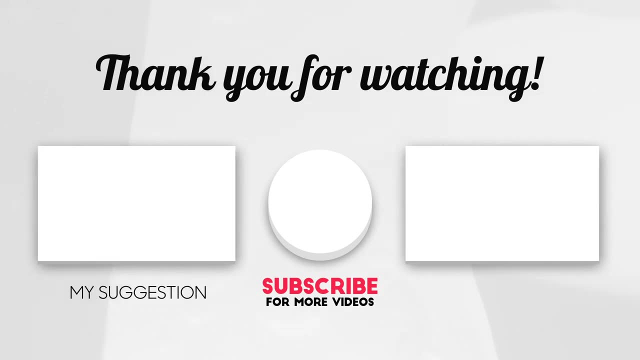 That's it for this video. I hope this video brought you value. If it did, please make sure to like and subscribe and I'll see you in the next one. Peace. 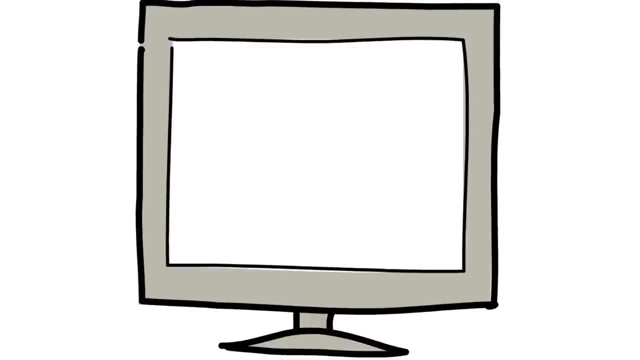 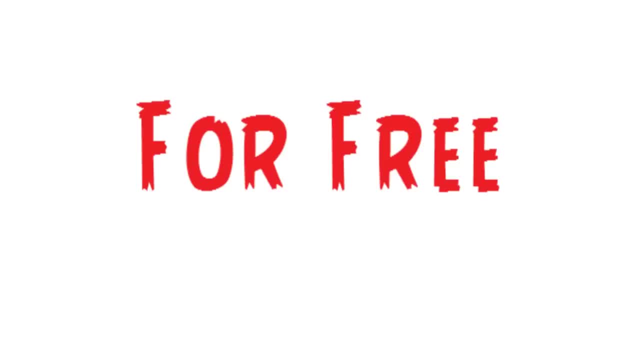 What's up, guys? this is Karat Code, and welcome back to a brand new video. In this video, I'm going to show you guys on how to learn programming for absolutely free. Now, before we start this video, there are some things you guys should know about this. First and foremost, you don't